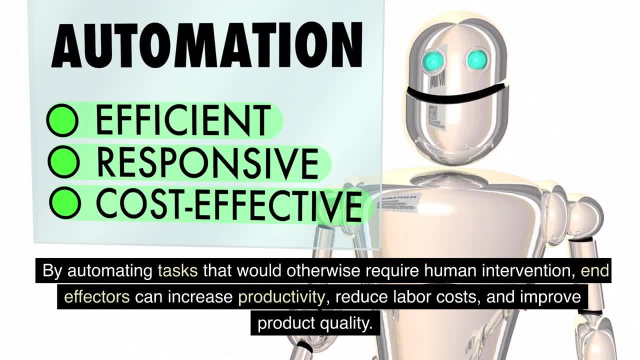 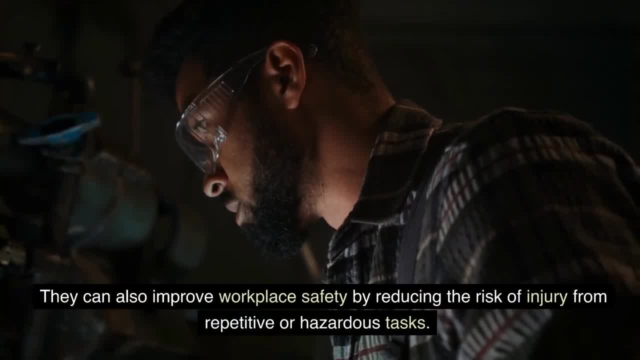 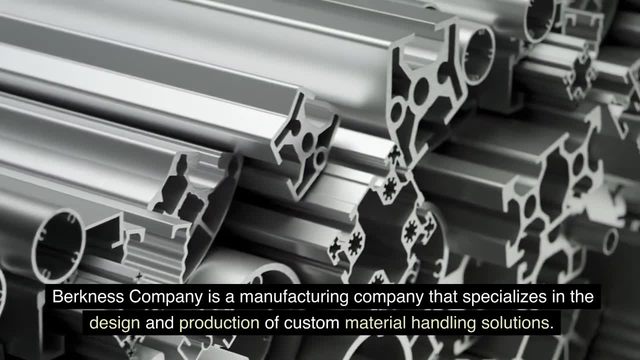 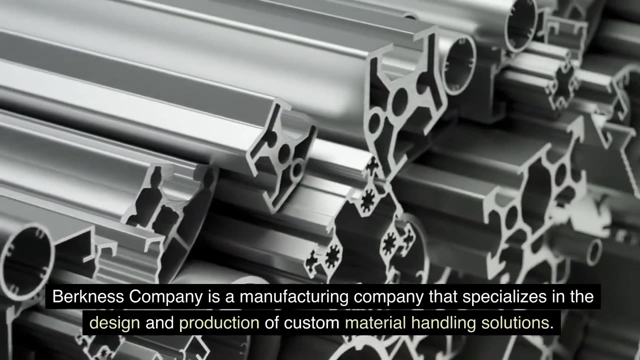 They can also improve workplace safety by reducing the risk of injury from repetitive or hazardous tasks. Berkness Company is a manufacturing company that specializes in the design and production of custom material handling solutions. As such end-effectors are a critical component of many of the company's products. 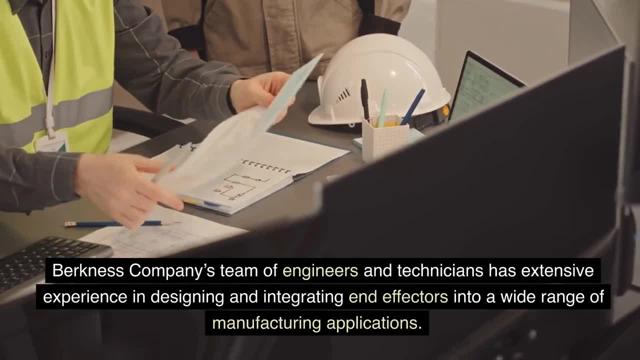 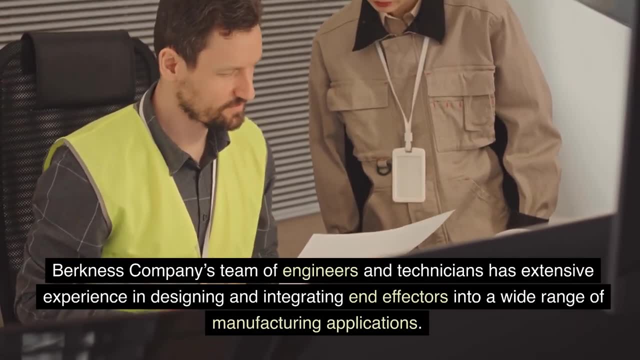 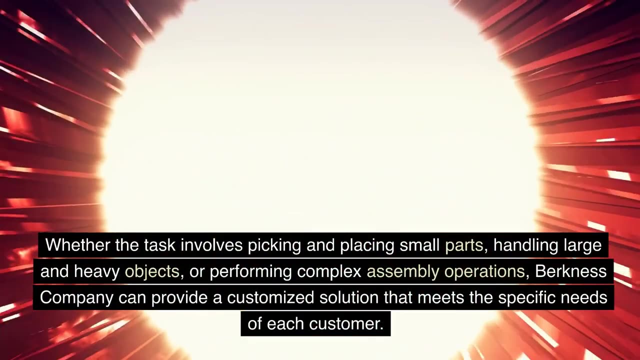 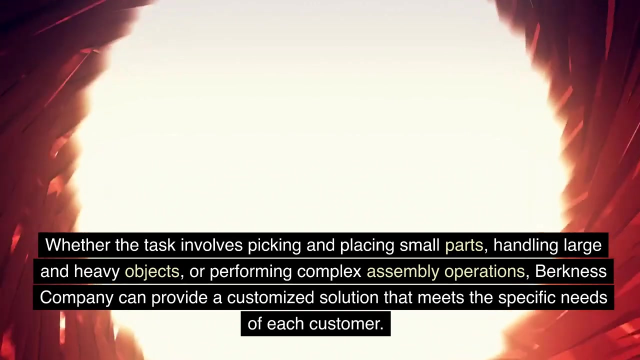 Berkness Company's team of engineers and technicians has extensive experience in designing and integrating end-effectors into a wide range of manufacturing applications. Whether the task involves picking and placing small parts, handling large and heavy objects, or performing complex assembly operations, Berkness Company can provide a customized solution that meets the specific needs of each customer. 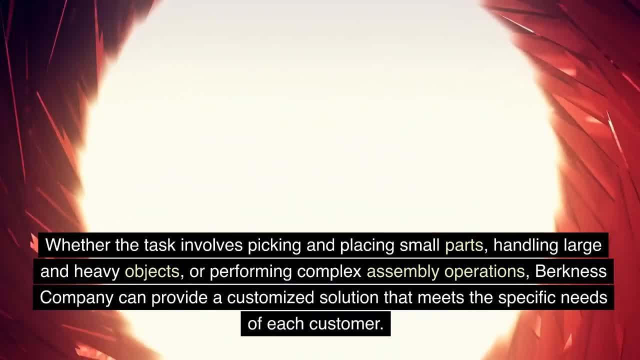 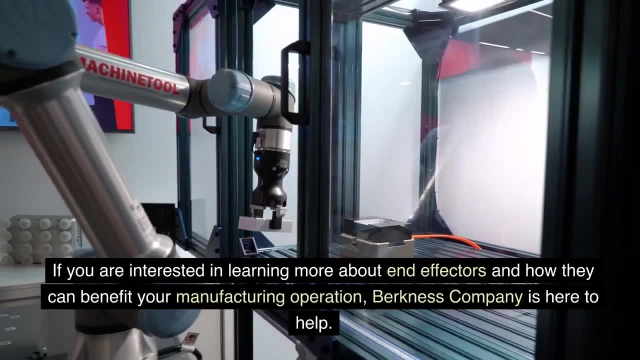 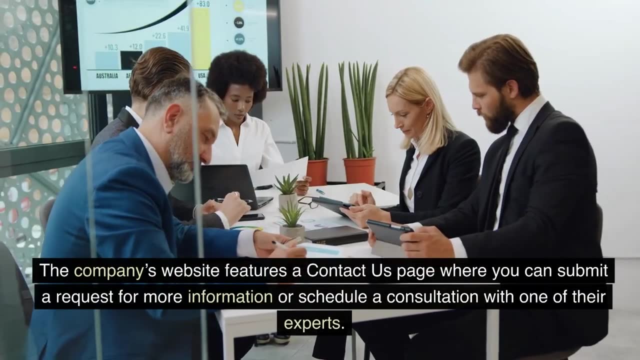 If you are interested in learning more about end-effectors and how they can benefit your manufacturing operation, Berkness Company is here to help. The company's website features a contact us page where you can submit a request for more information or schedule a consultation with one of their experts. 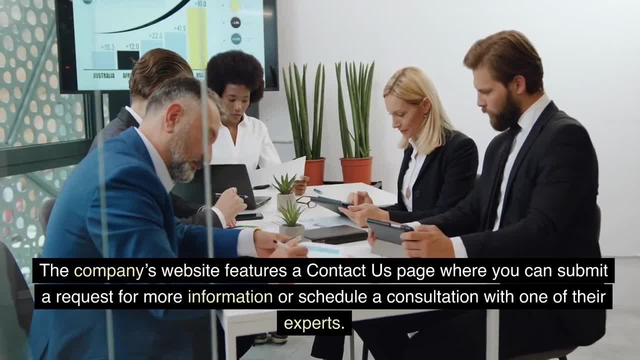 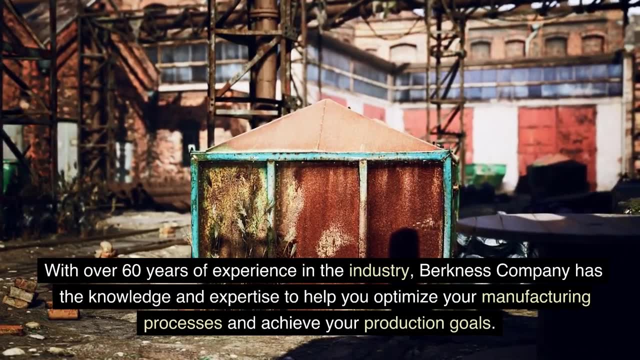 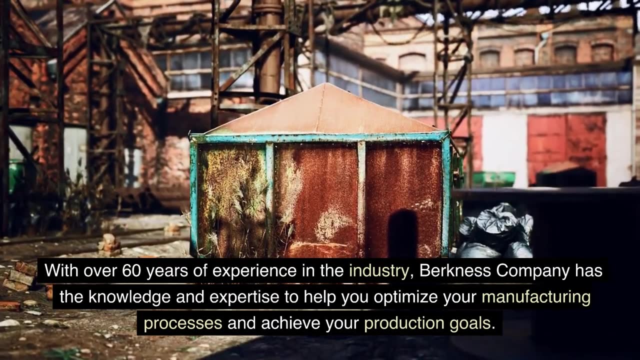 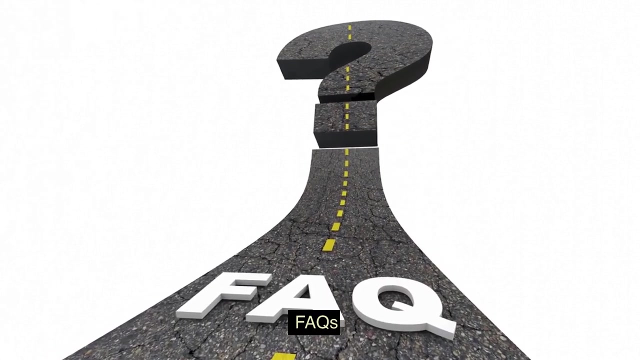